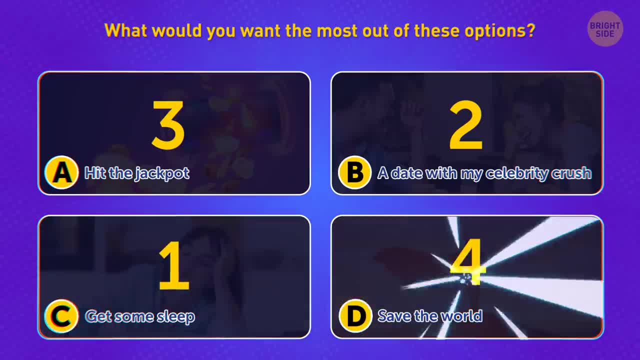 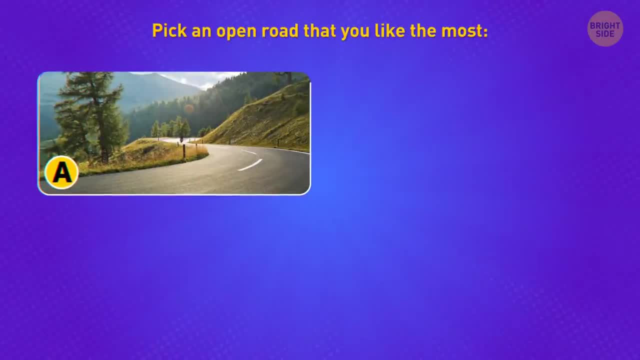 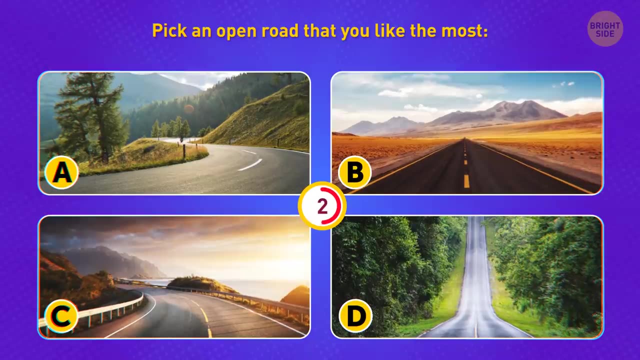 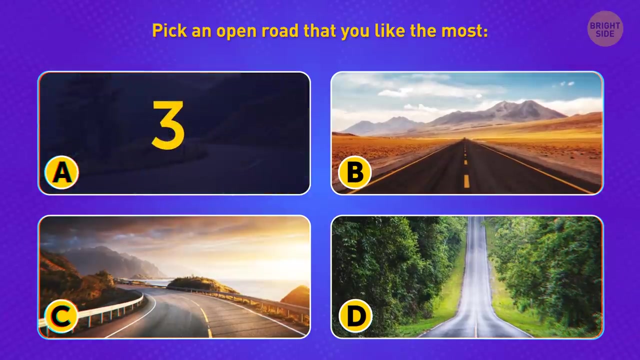 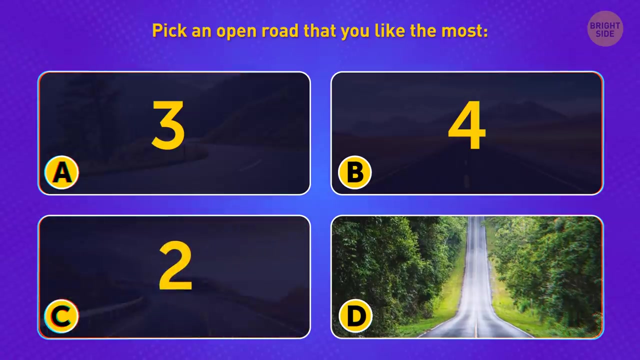 Card C costs one star. Option D brings you four points. Pick a door, Pick an open road that you like the most. The mountain highway brings you three stars. If you chose the desert, add four points to your score. Sunrise highway costs two stars. The road through the rainforest brings you one point. 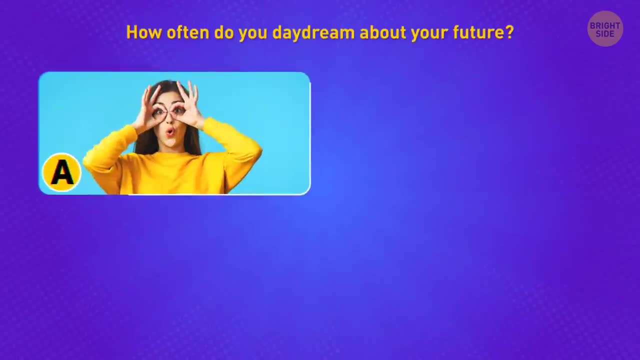 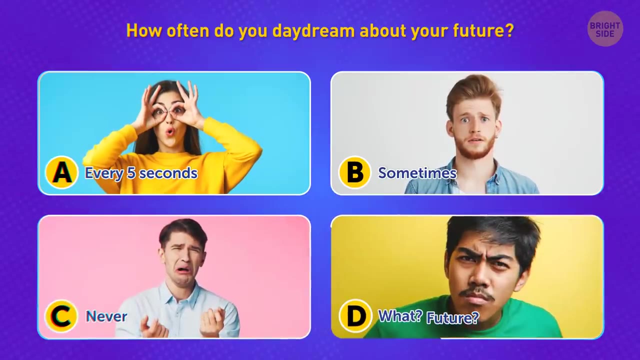 Option D brings you three stars. If you chose B, add four points to your score. How often do you daydream about your future? Every five seconds, Sometimes Never Future- I don't even know this word. Option A adds one star to your score. 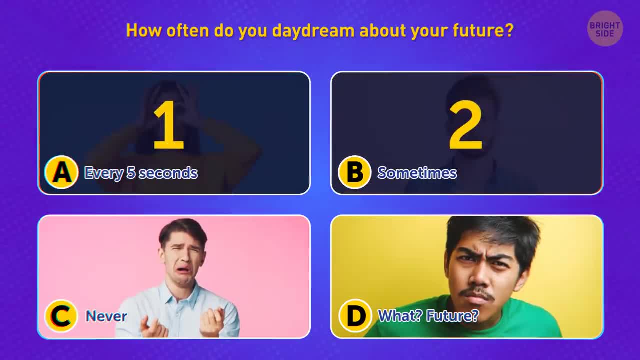 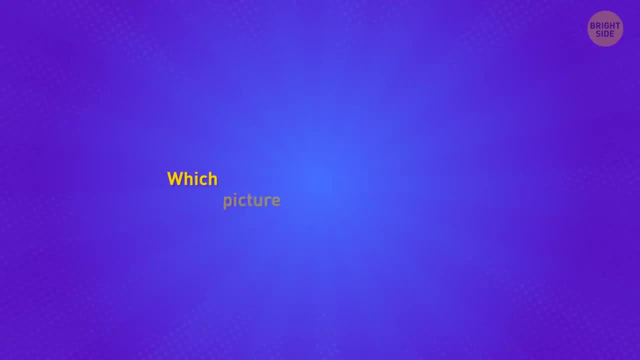 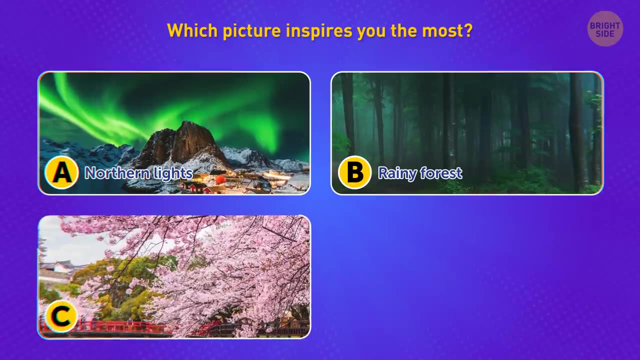 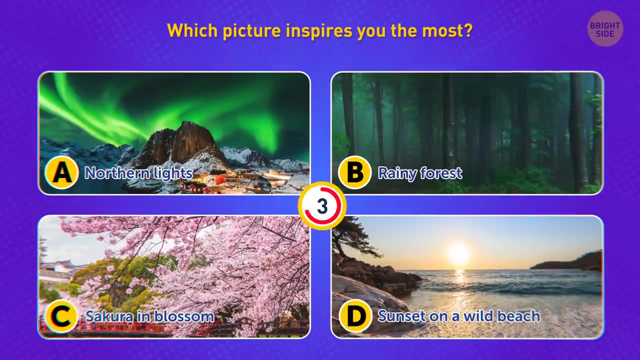 B brings you two points. If your choice is C, it's worth three stars. Option D brings you four points. Which picture inspires you the most? Northern lights, Rainy forest, Sakura in blossom Sunset on a wild beach. If your choice is Option A, add four stars to your basket. 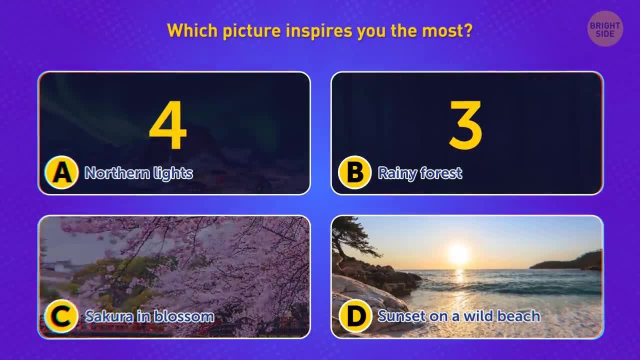 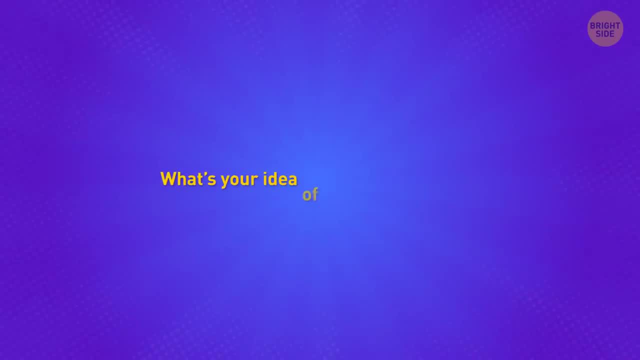 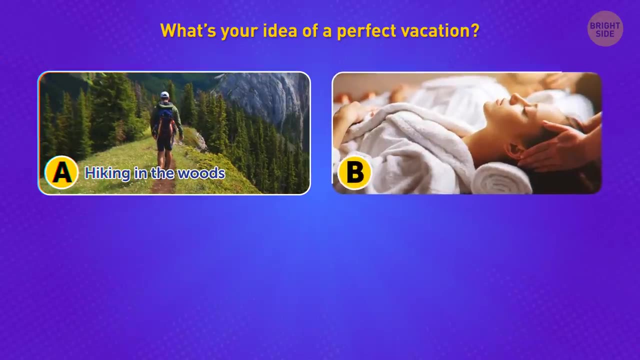 Option B is worth three stars, Option C brings you two points And Option D is worth one star. What's your idea of a perfect vacation? Hiking in the woods by myself, I love to be alone. Luxury spa with my besties, Because we're worth it. 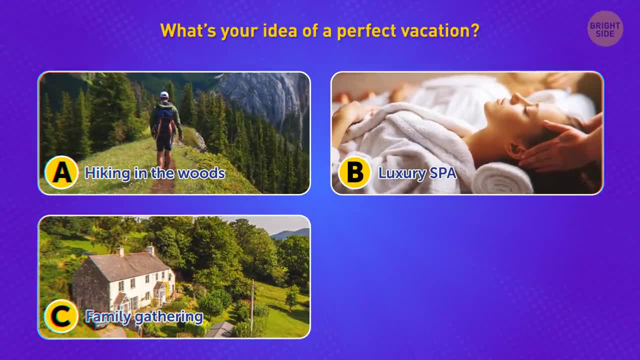 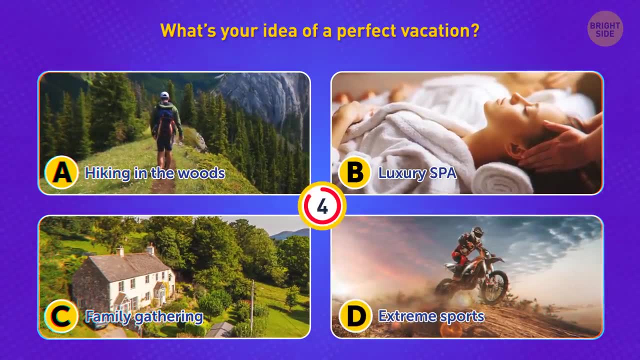 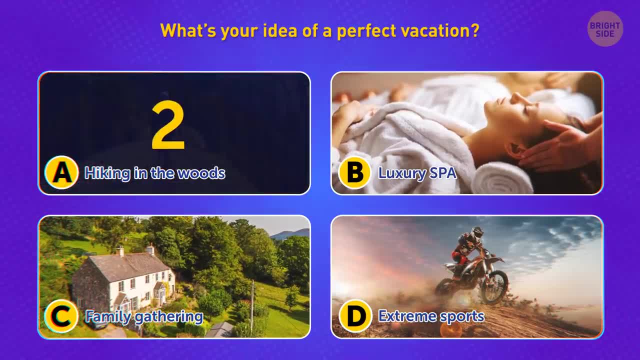 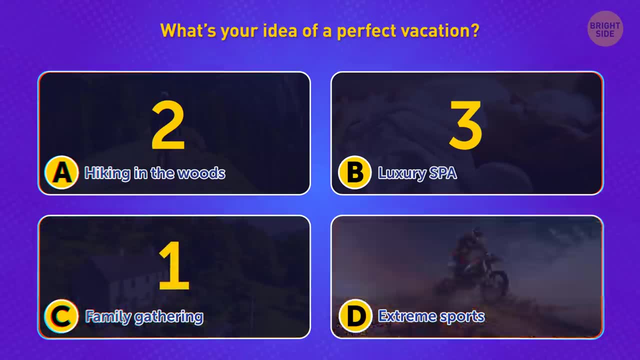 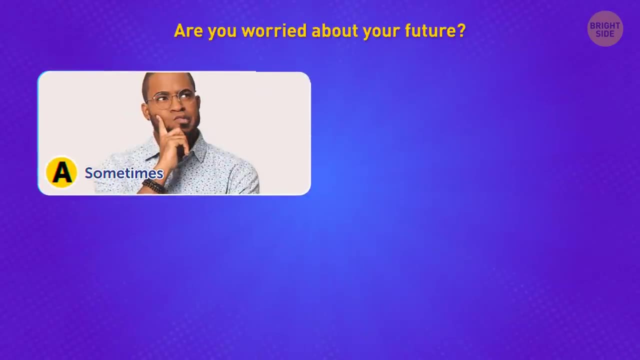 Card A brings you two stars. Card B adds three points to your score. If you chose C, add one star to your basket. Option D brings you four points. Are you worried about your future? Sometimes I like to have a plan B. 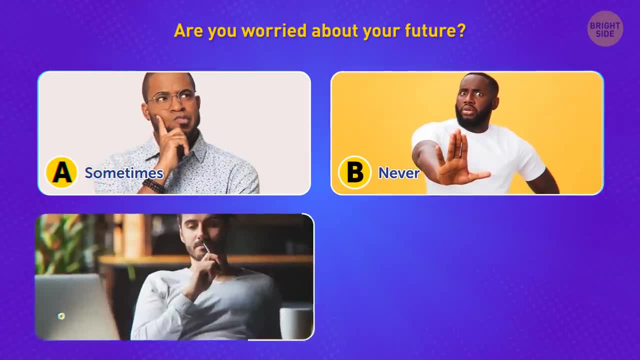 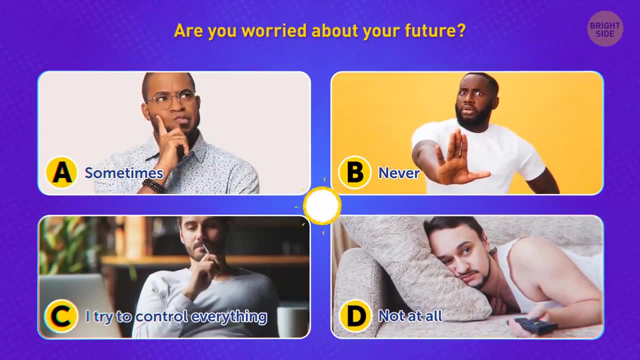 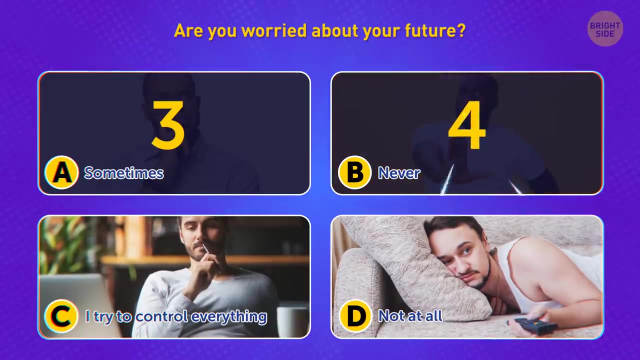 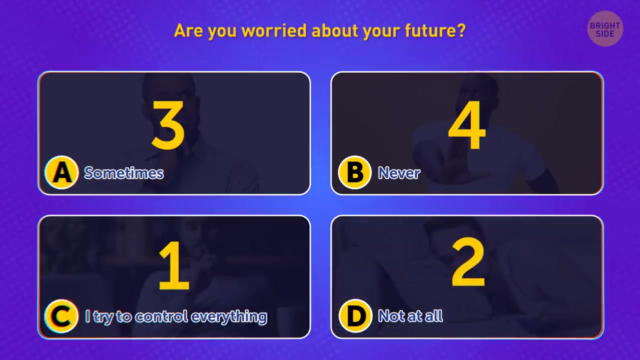 Never I live in the moment. Always, Always, always. i try to control everything. nope, i spend all my time regretting my past. if you picked option a, add three stars to your score. option b brings you four points. option c is worth one star. if d is your choice, it brings you two points. what's your most? 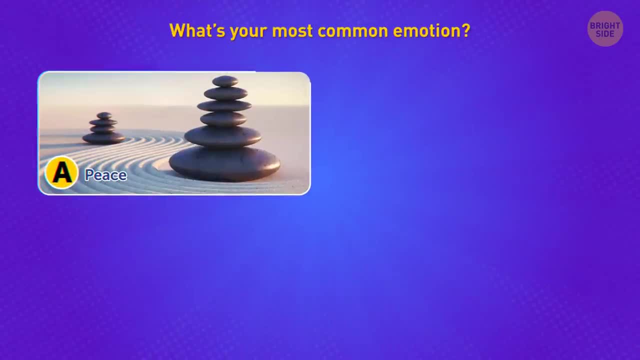 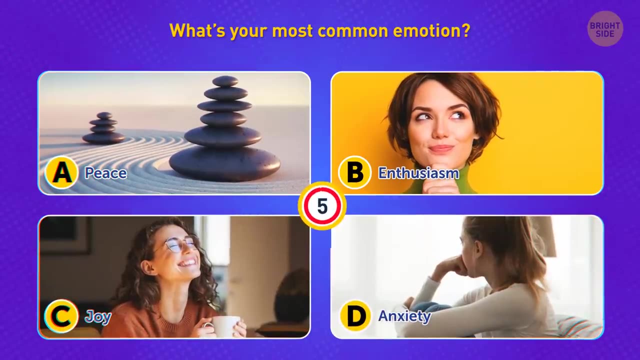 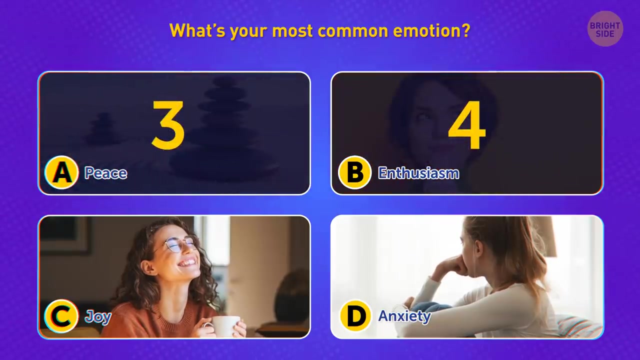 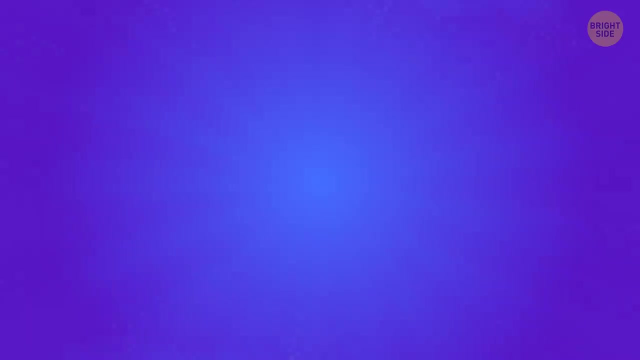 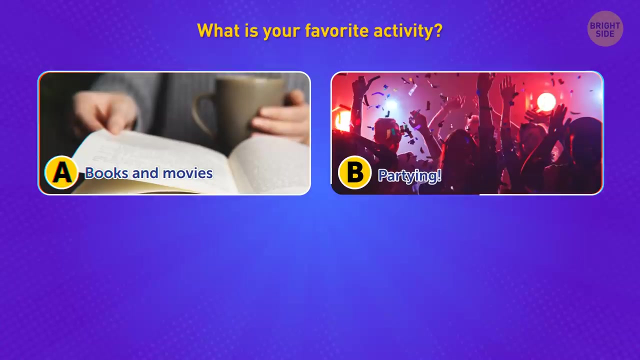 common emotion: peace, enthusiasm, joy, anxiety. option a brings three stars to your score. if you chose b, add four points to your basket. option c brings you one point and option d is worth two stars. what is your favorite activity? reading books and watching movies, partying with friends and meeting new people, studying and developing new skills. 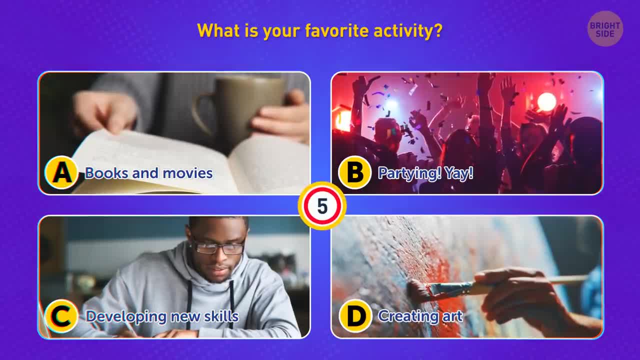 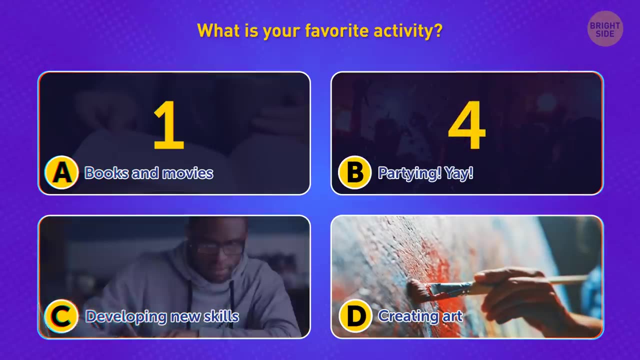 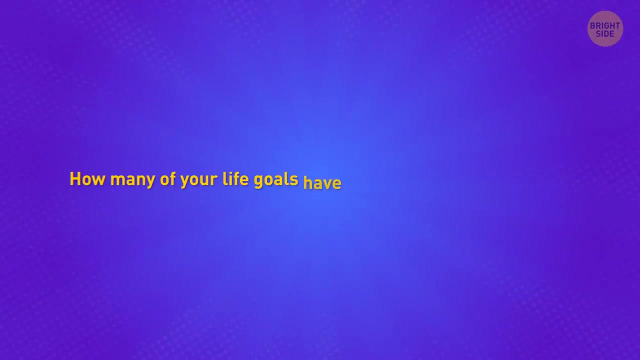 creating art and sharing content. if you picked option a, add one star to your score. Option B brings you 4 points. Option C is worth 3 points. Option D brings you 2 points. How many of your life goals have you already accomplished? Zero. My to-do list for this life is 50% completed. All of them. I want it, I got it. I don't set any goals. The universe knows better. If you chose A, add one star to your score. 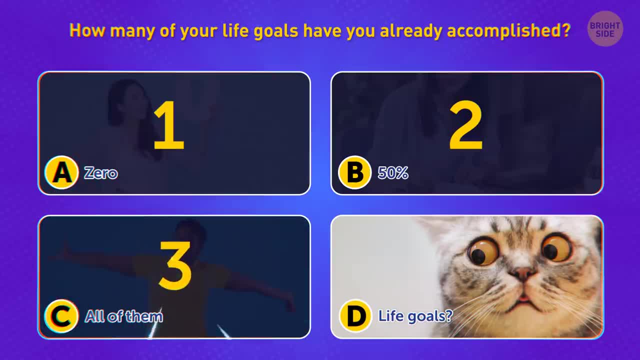 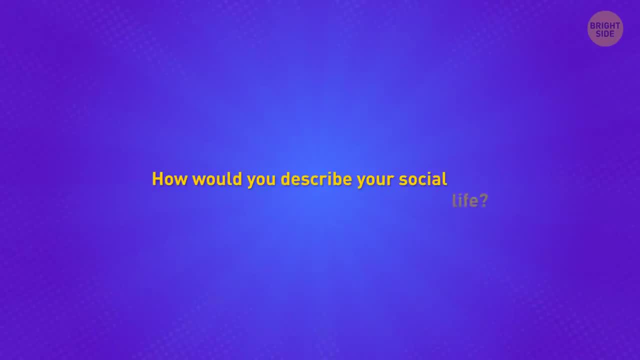 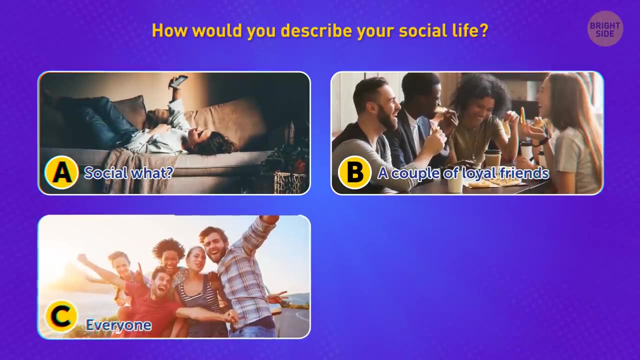 Option B brings you 2 points. C is worth 3 points. Option D brings you 4 points. How would you describe your social life? Social, what I have? a couple of loyal friends. Every human being is my friend. My friend circle is always changing. 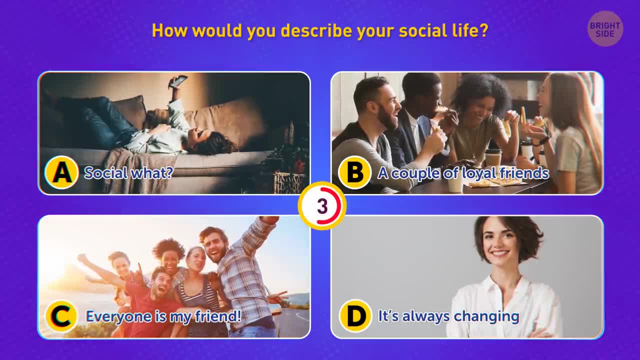 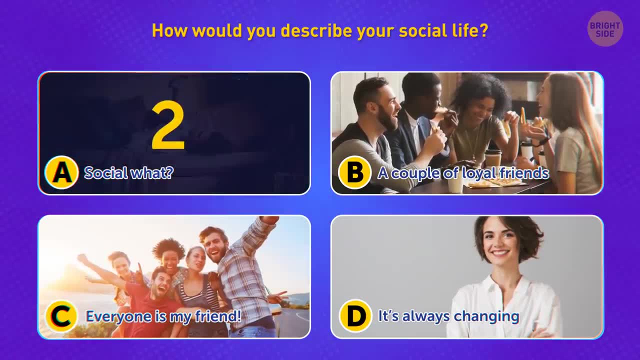 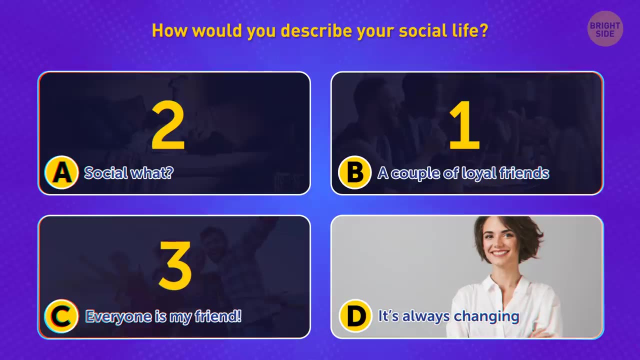 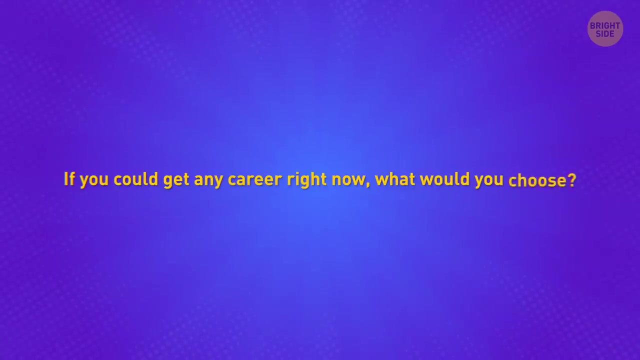 I love you. Card A adds 2 stars to your score. If you picked option B, take 1 star. Did you pick option C? Award yourself with 3 stars. Option D brings you 4 points. If you could get any career right now, what would you choose? 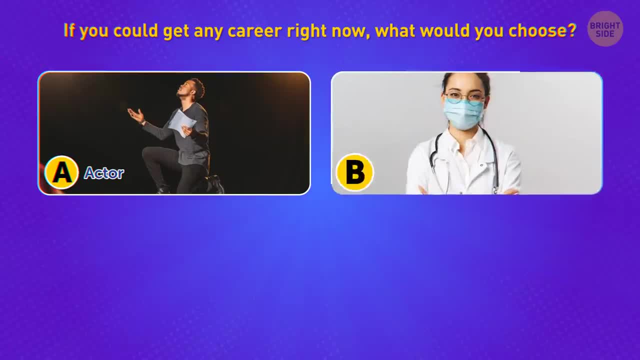 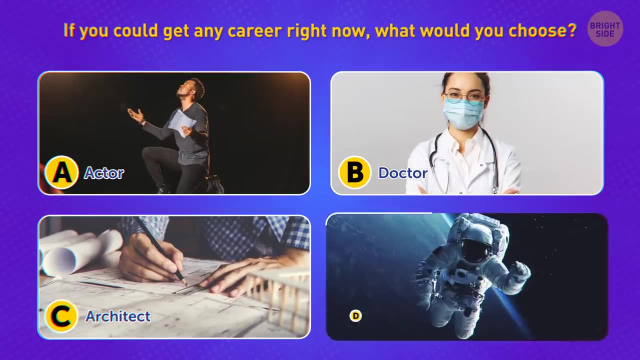 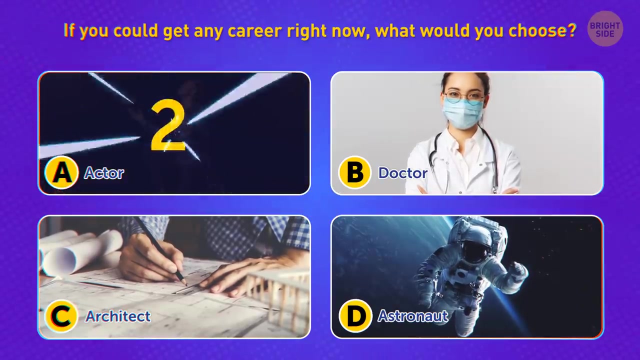 Actor: I love to be the center of attention. Doctor: I love to be the center of attention. Character: I want to help others. Architect: I like to create spaces. Astronaut: I'd love to discover new worlds. If you chose A, add 2 stars to your score. 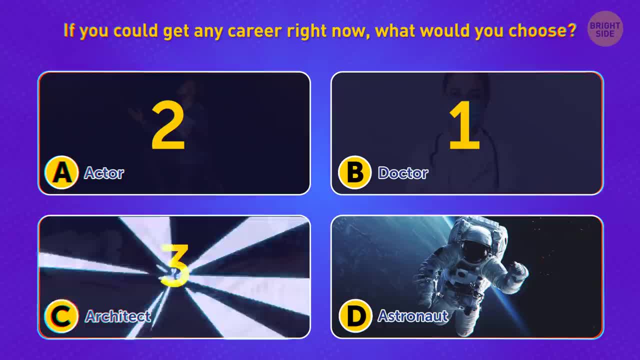 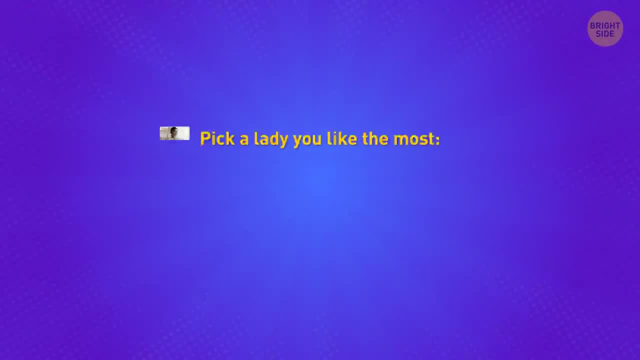 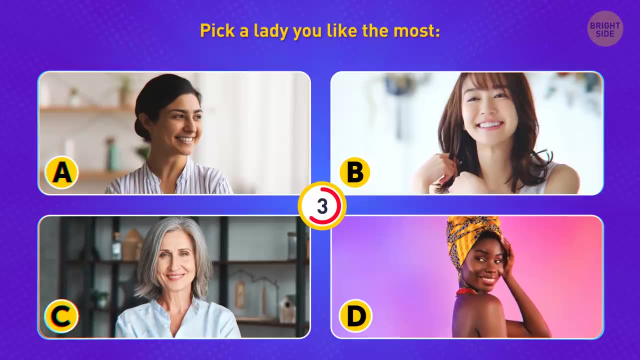 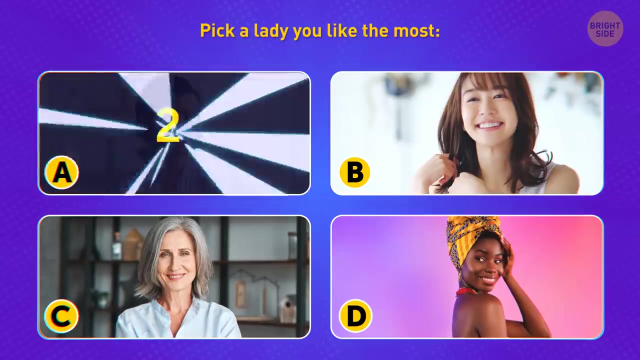 Option B brings you 1 point. C costs 3 stars. Option D brings you 4 points. Pick a lady you like the most. If you picked lady A, grab 2 points. Option B adds 1 star to your score. 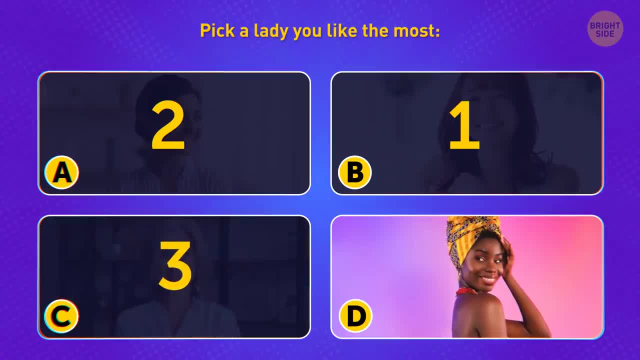 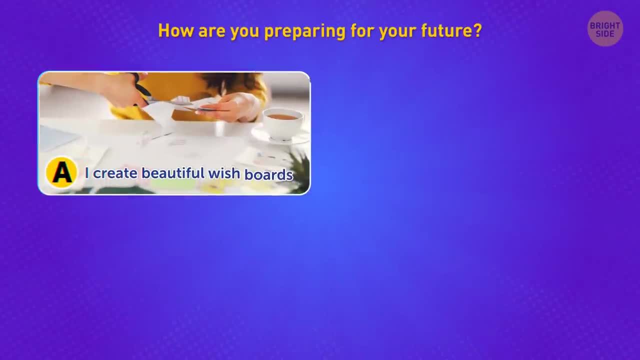 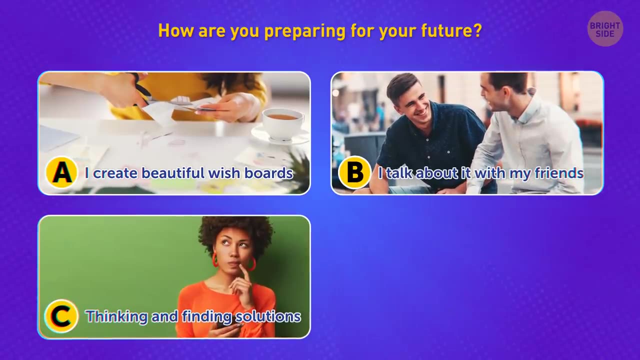 Option C brings you 3 stars And answer D brings you 4 points. How are you preparing for your future? I create beautiful wishboards- I just talk about it with my friends, Thinking and finding solutions to my current issues. I take it step by step every day. 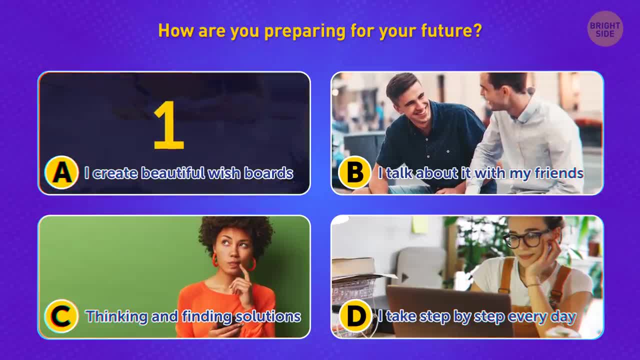 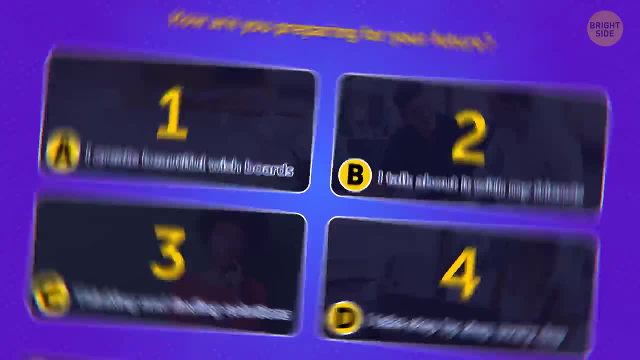 If you picked option A, add 1 star to your score. Option B brings you 2 points. 3 will cost 3 stars. Option D brings you 4 points. Option E brings you 9 points. Sporting the car Options A brings you 4 points. 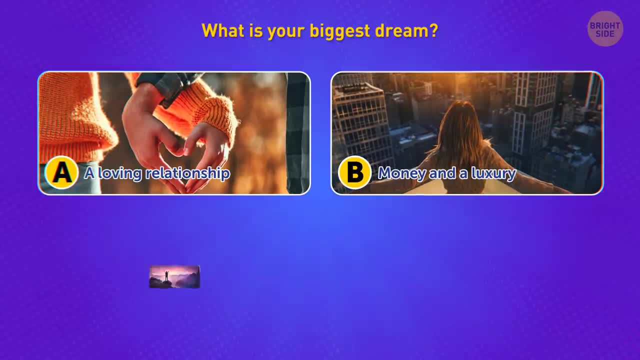 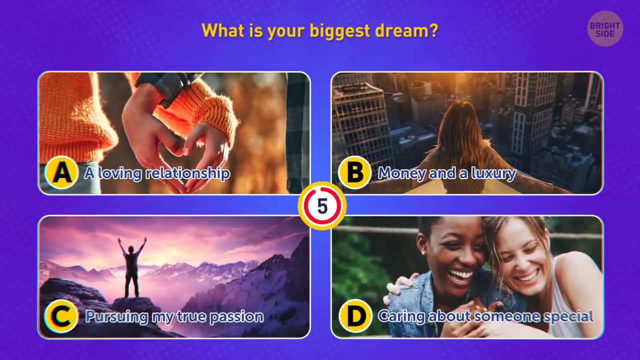 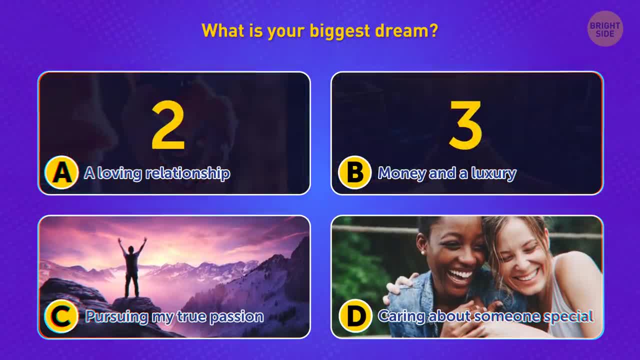 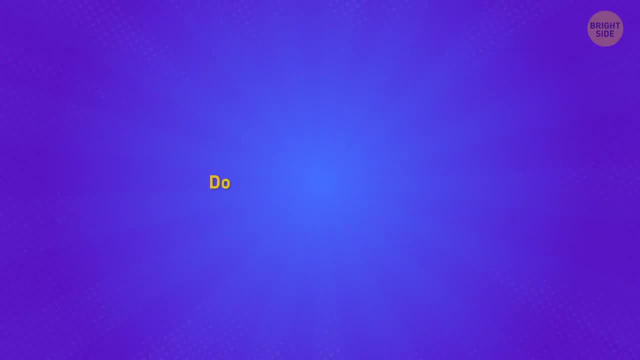 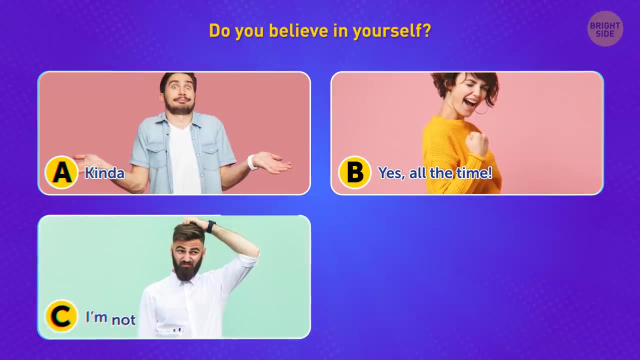 A loving relationship. B Brings you three points, C Costs four stars, And if your choice was option D, you get one point. Do you believe in yourself? Kinda Yes, all the time. Nope, I'm not exactly perfect, bro. 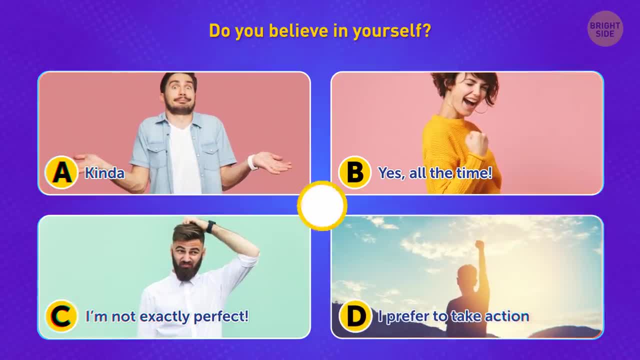 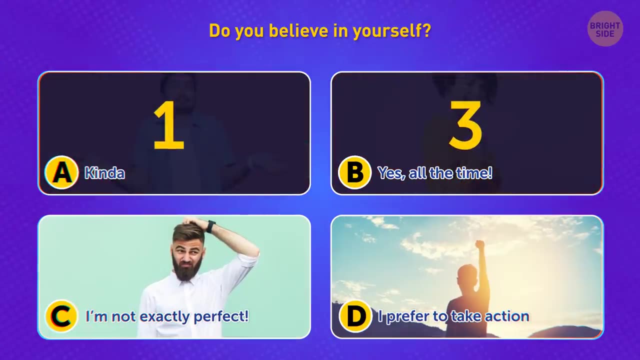 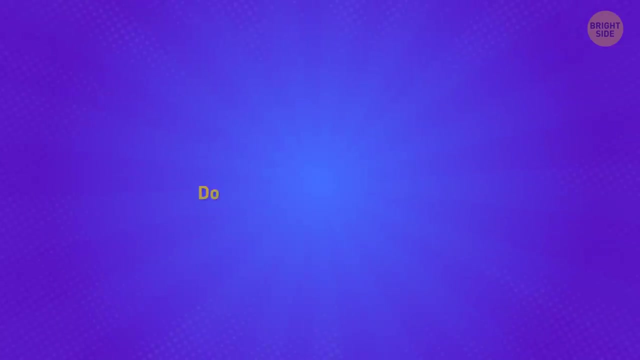 I prefer to take action and not think about that. If you chose A, add one star to your score. Option B brings you three points. Option C is worth two stars. Option D is worth three points. Do your parents support you? Nope, I'm on my own in this world. 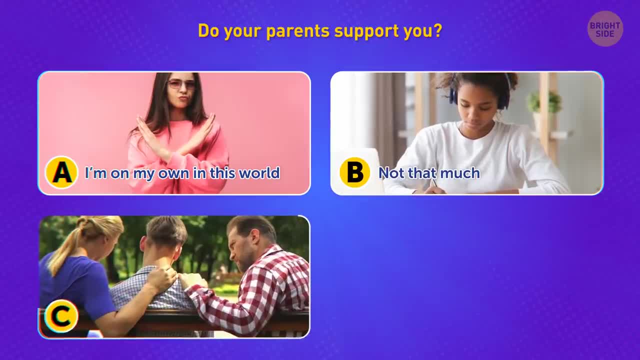 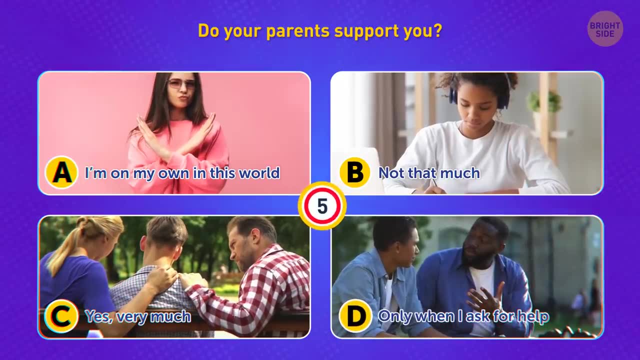 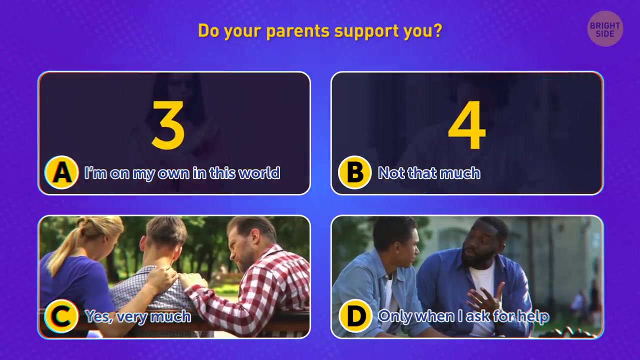 Not that much. they got their own lives. Yes, my happiness means everything for them, Just a little when I ask for help. If you chose A, add three stars to your score. Option B brings you four points. Option C costs one star. 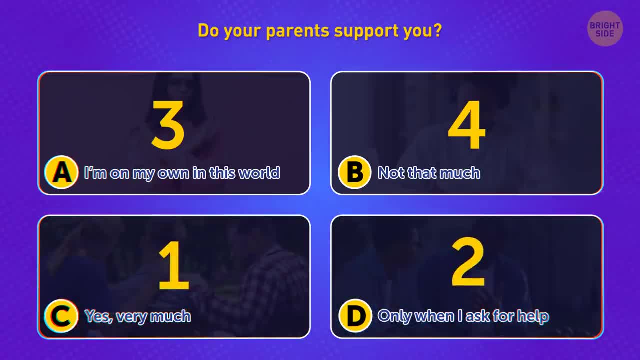 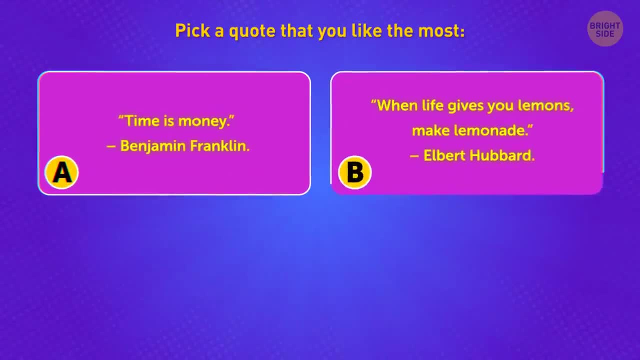 Finally, option D brings you two points. Pick a quote that you like the most. Time is money. Benjamin Franklin, When life gives you lemons, make lemonade, Albert Hubbard. If you want to be happy, be Leo Tolstoy. 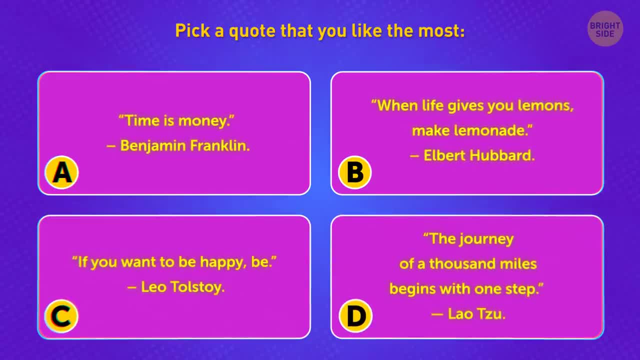 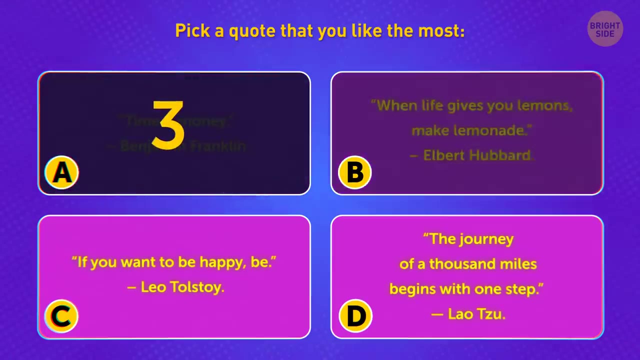 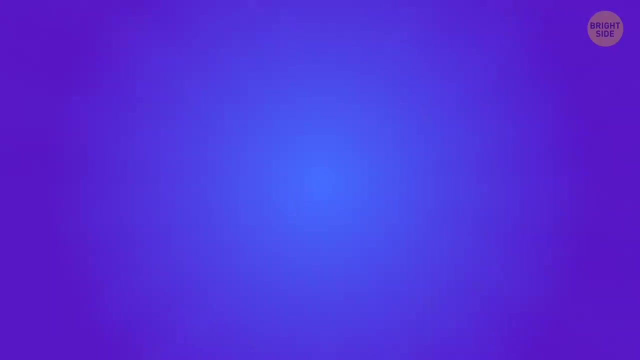 The journey of a thousand miles begins with one step. Lao Tzu. Option A adds three stars to your score. Option B brings you two points. If you chose C, take one star. Option D brings you three points, Which sounds most like you. 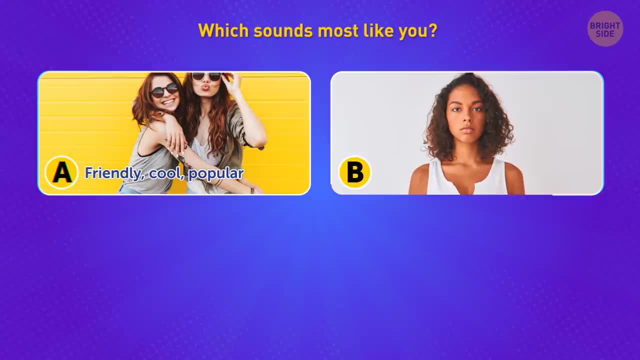 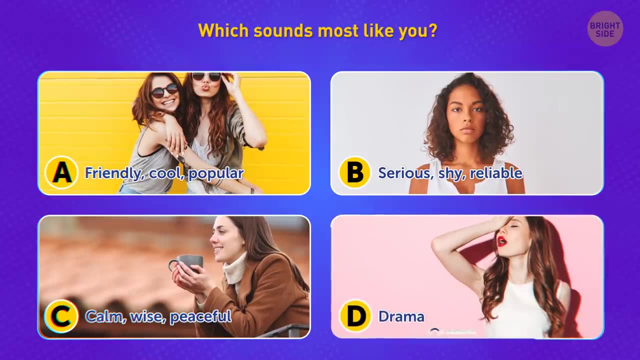 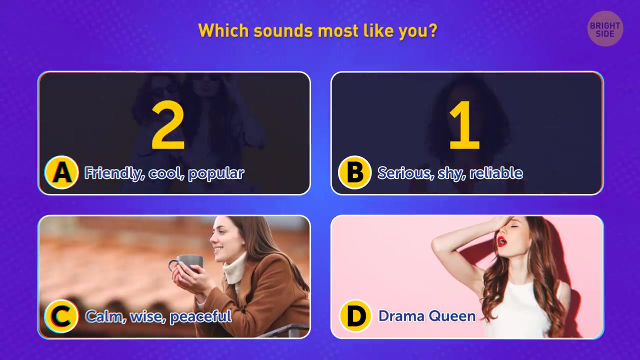 Friendly, cool, popular, serious, shy, reliable, calm, wise, peaceful, drama. queen Card A adds two stars to your score. Option B brings you one point. If you chose C, grab three stars. Option D brings you four points. 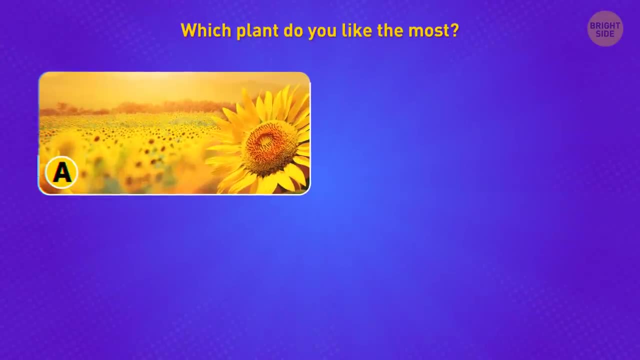 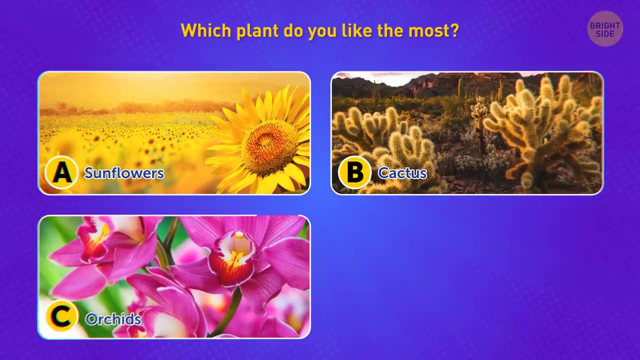 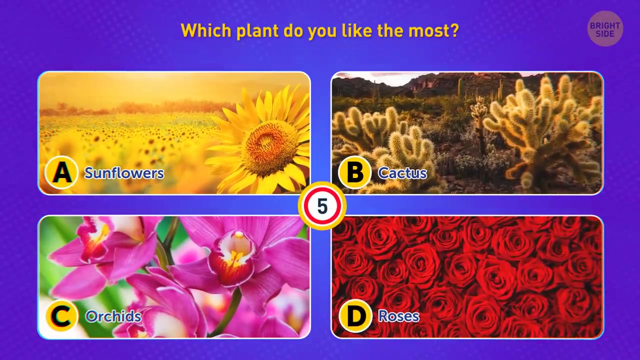 Which plant do you like the most? Sunflowers always warm my heart. Cactus: We have a lot in common. Orchids: I love their sophisticated beauty. Roses: What could be better than the classics? Card A Adds four stars to your score. 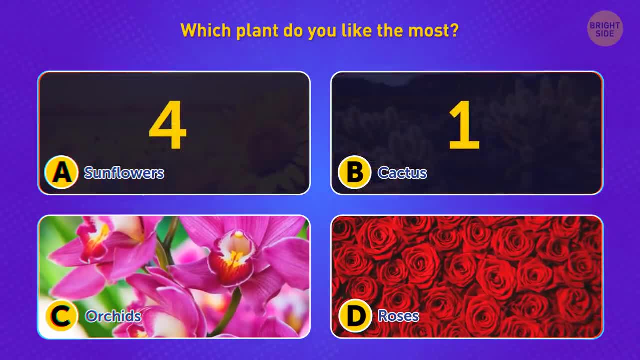 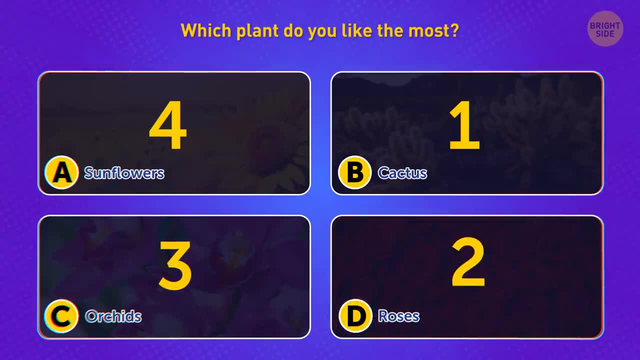 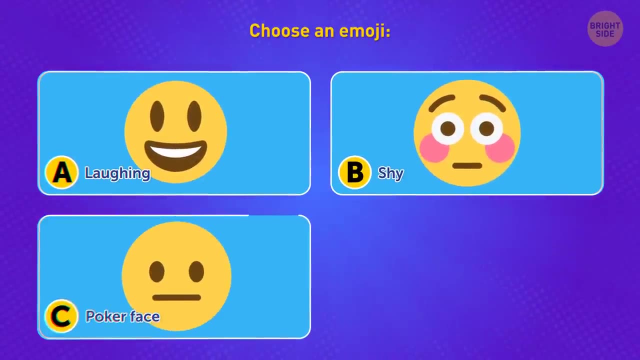 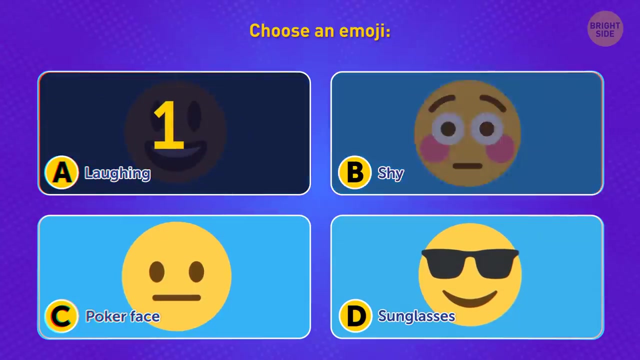 Option B brings you one point. If you chose C, three stars are coming your way. Those who went for D get two points. Choose an emoji: Laughing: Shy Poker face Sunglasses. A Adds 1 star to your score. B Brings you 2 points. 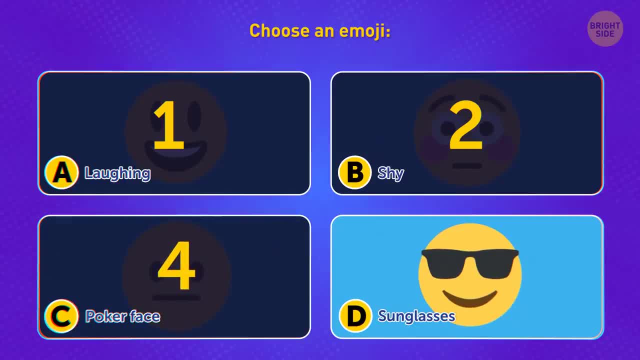 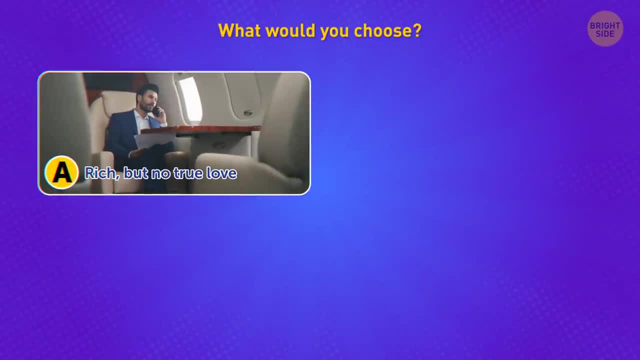 Option C Adds 4 stars to your score. D Brings you 3 points. What would you choose? Get rich, but never find true love. Find true love, but never get rich. I'm already rich. Where's my soulmate? 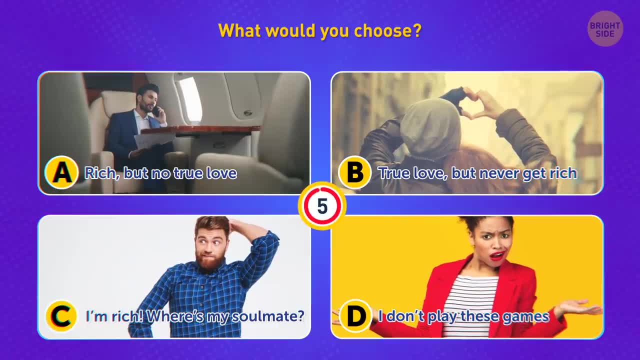 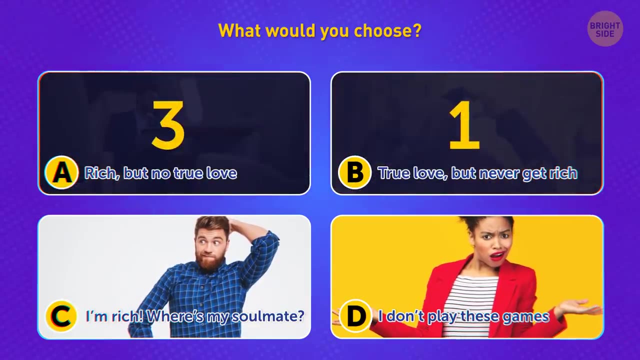 I don't play these games, bro. Card A Adds 3 points to your score. Option B Brings you 1 point. If you chose C, grab 2 stars. Option D Brings you 4 points. Ready for the results. 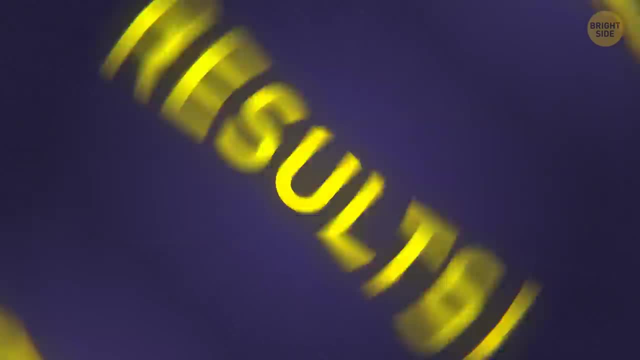 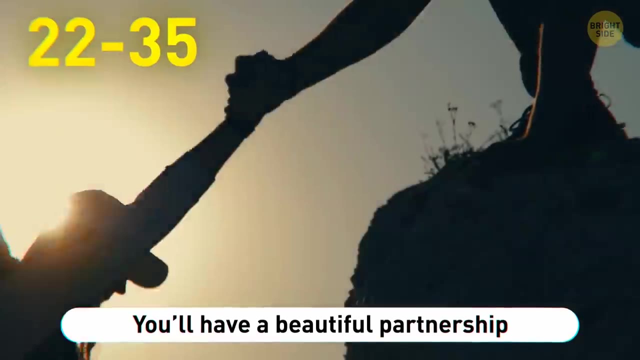 Make sure you sum up your score correctly. Let's go 22 to 35 points. Your future is about having a beautiful partnership. You'll make it with the right person who shares your life goals and values. Together you'll build the life of your dreams, step by step. 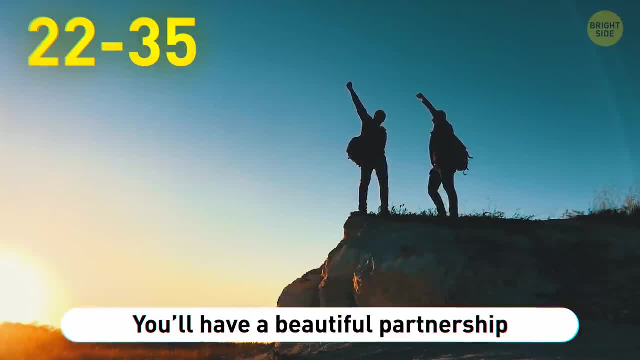 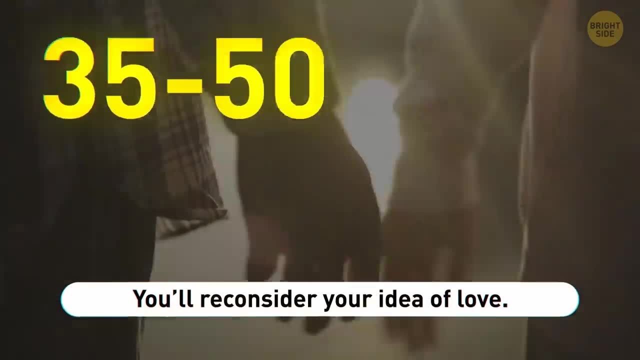 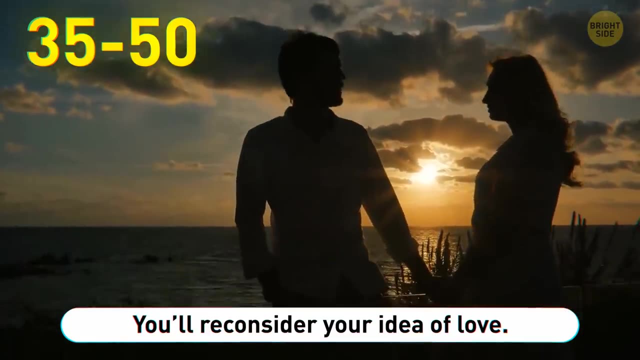 This journey will bring joy and satisfaction. every day, 35 to 50 points. Your future will force you to reconsider your idea of love. You'll meet your true soulmate when you least expect it. Your heart will recognize them at first. This person will inspire you to become a better version of yourself every day. 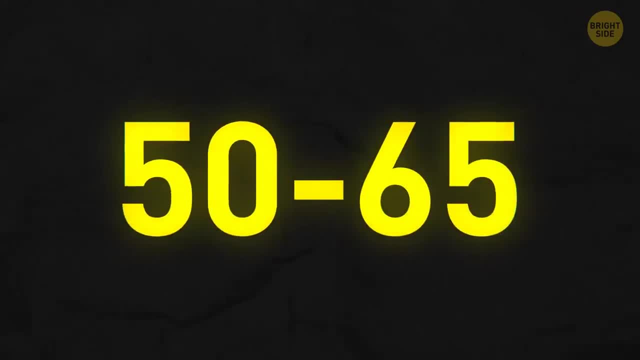 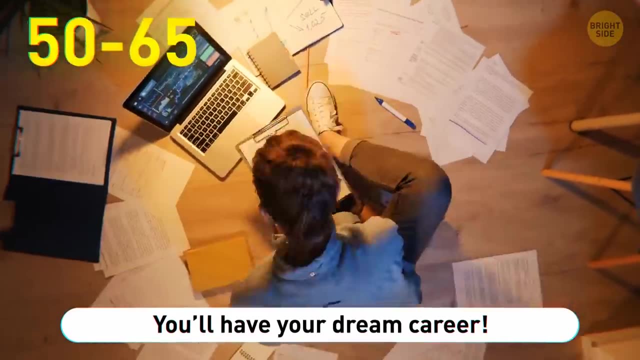 This experience will be beautiful. 50 to 65 points Congratulations. Your future is about having a beautiful relationship. You're pretty determined and you can make it if you really want it. Stay focused and know that the stars are on your side. 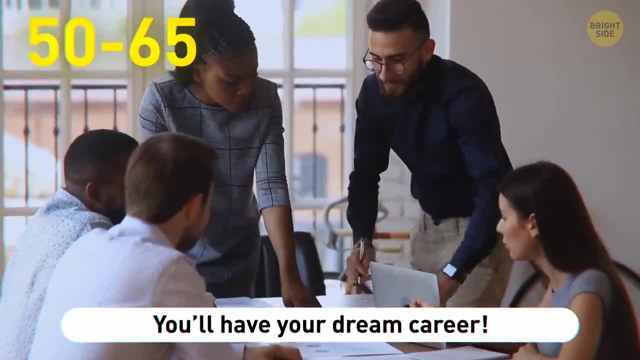 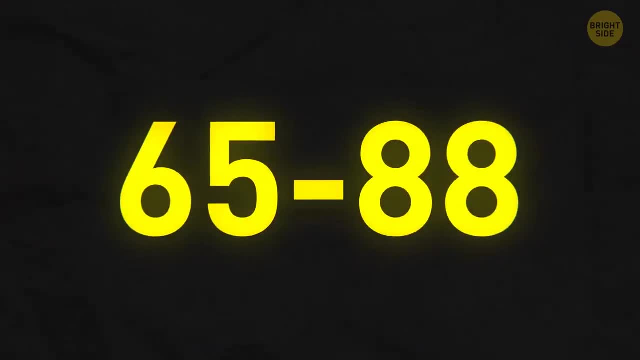 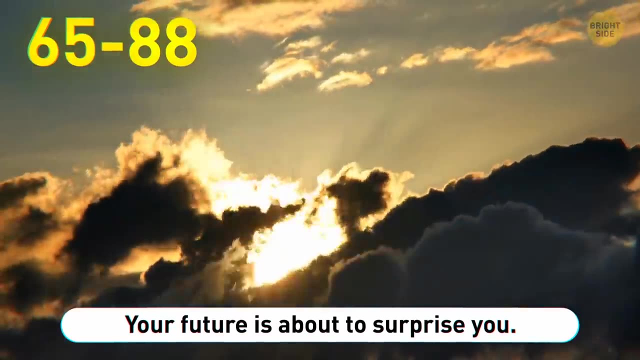 You may even outgrow your original dream and switch to building a community of like-minded people to share your experience and give them a sense of purpose. 65 to 88 points: Your future is about to surprise you. The chances to make your biggest dreams come true are very high.